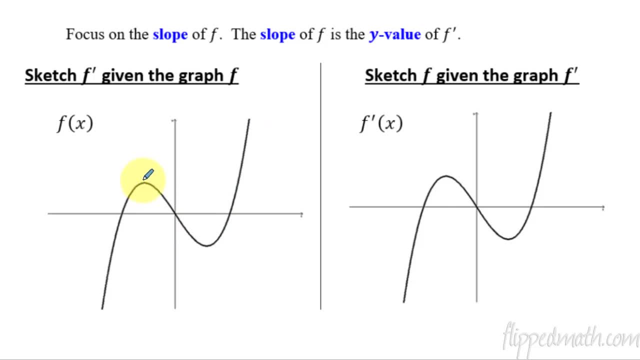 some things I already know about the slope along F. So let's think about, right here: I know that the slope is zero, right there at that maximum point, And here, at the minimum point, I also know that the slope is going to be zero. 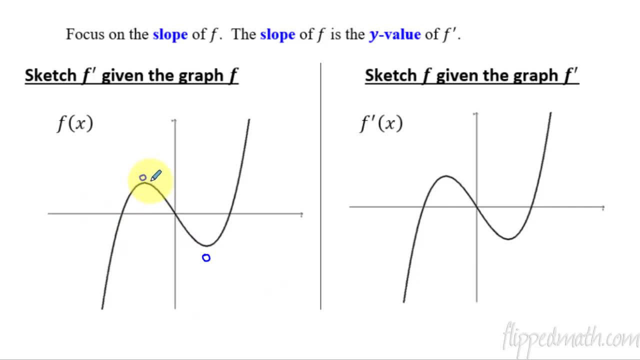 Here the slope is close to zero, but it is going to be negative. so it's really small negative. Here it's really small positive. And then same here. Here it's really small negative, really small positive, It's just barely positive. But 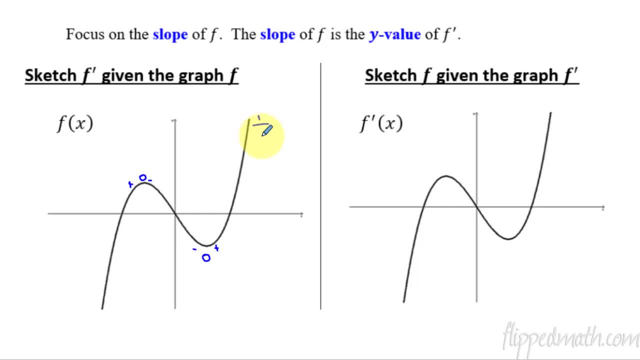 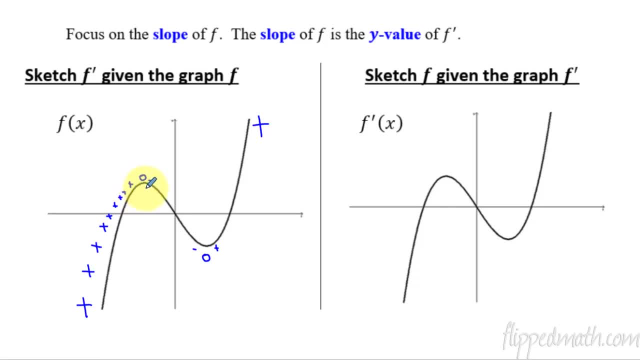 just gets really, really tiny. So it's still positive, but it's barely positive. And then it hits zero, and then it's negative, and then more negative, and more negative, And then, right here, at the point of inflection, is where it's the most negative. And then the negative starts to get not quite so negative not. 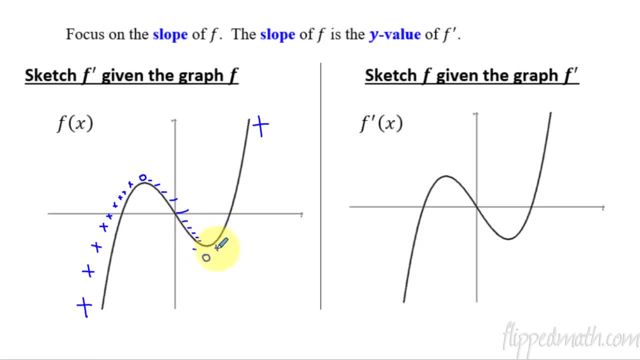 quite so negative until we get back to zero. And then same here. So it's a very, very barely positive, and then larger positive, larger positive, larger positive, and so forth till we get to the most positive of all the graph. Okay, so the reason I did that is because I want you to think what the 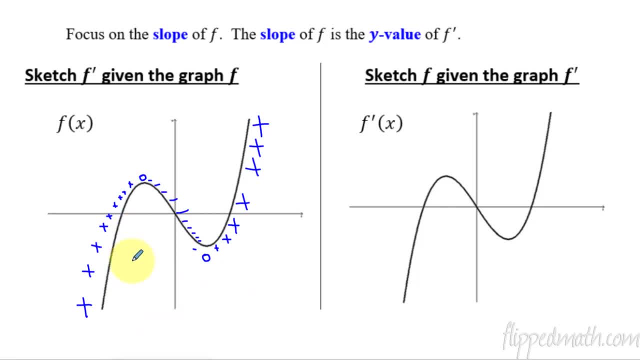 derivative graph would look like based on this. Let me switch colors. That way you can really see what's going on here. So let's start with what we know, and that is the zero. So I'm gonna put a zero right there, and my f prime will also. 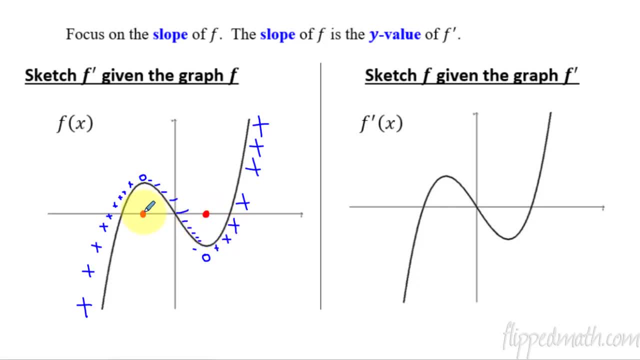 have a zero there. And now what else do we have going on In between these? see how this is all minus, minus, minus minus. So that means the y values of f prime are all negative. The y values of f prime will all be. 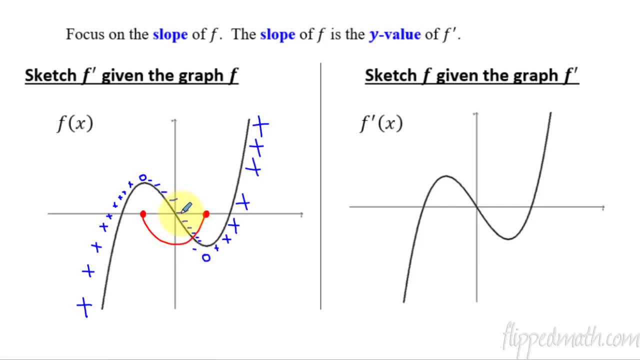 here Like that. Now, here's where it's the most negative, at this point of inflection, and that's why that's my minimum point, Because it's the most negative point. the point of inflection will also give you a zero of of f prime. 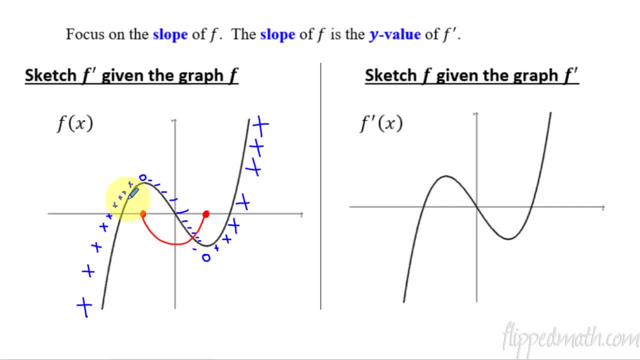 So it all starts connecting together This f, f, prime, f, double prime. And now here we're going to have this graph go all the way up like this. So it's kind of like this is basically just a parabola, right? Yep, we're going up like this, Okay. 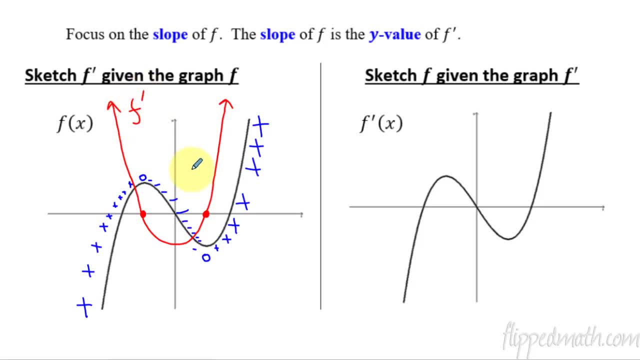 so now think about what we've done. This in red is f, prime, Okay, the original one in black is just f, And we have positive slope, really positive slope, getting really close to zero, Then negative slope, zero, again positive slope. And if you look at the red, the y values start. positive The y. 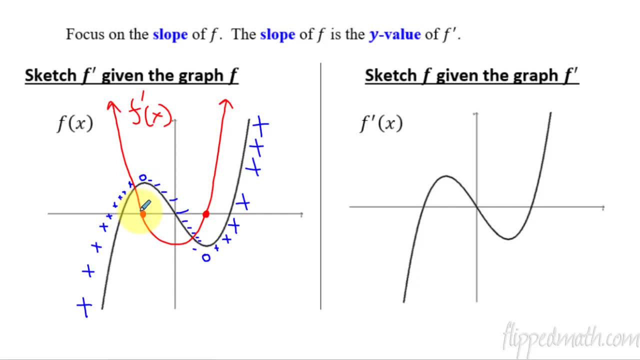 values get smaller, smaller. they're still positive, but they get smaller, really tiny, then zero, And then they're barely negative and then more negative, more negative, back to zero, and then positive, positive, positive. Okay so 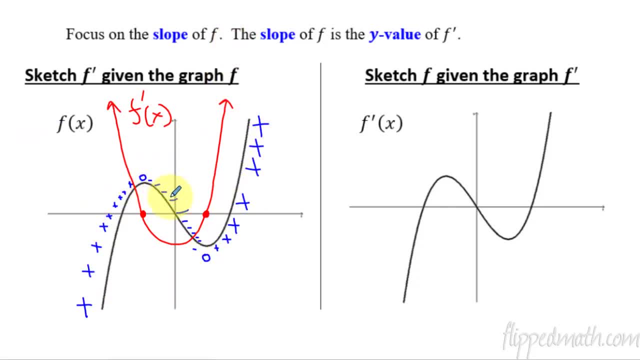 that's how you start with f, If you need to just label what the slope looks like and then that might help you sketch the graph. Okay, next up, f, prime. So notice, I gave you the exact same graph. It's this cubic type of a function. It's the exact. 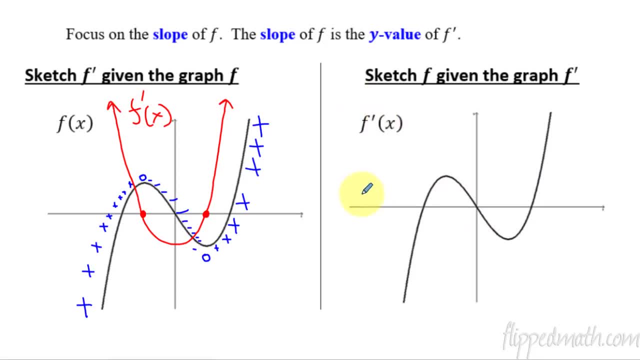 same graph, but this time I labeled it as f prime. So what would happen now If I say this is f prime, let's go the other direction. So let's see, we've been doing this, this whole unit, right? We've been trying to figure out a bunch of these. 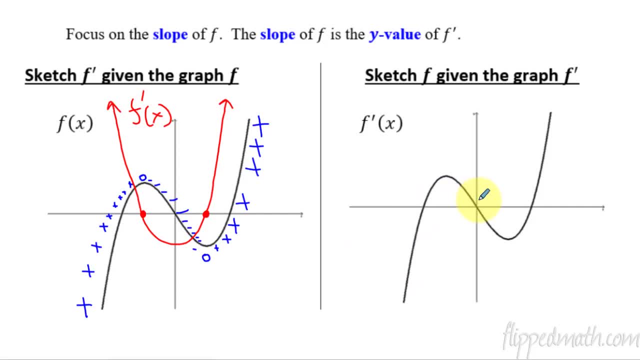 things with where f prime changes signs from negative to positive, positive to negative, So that should be a little bit familiar to you already. Let's just label then what we know. We know it's going changing from negative to positive, and when f prime changes from negative to positive, we have a minimum. 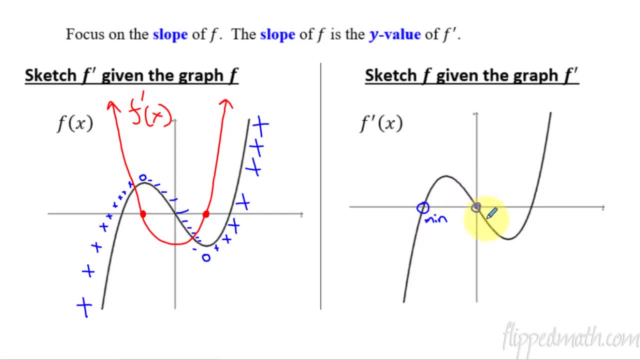 And when it changes from positive to negative, we have a max, And when it changes from negative to positive, we have a minimum again. And what else do we know? Oh, we know when f prime prime, so when the derivative of f prime changes. 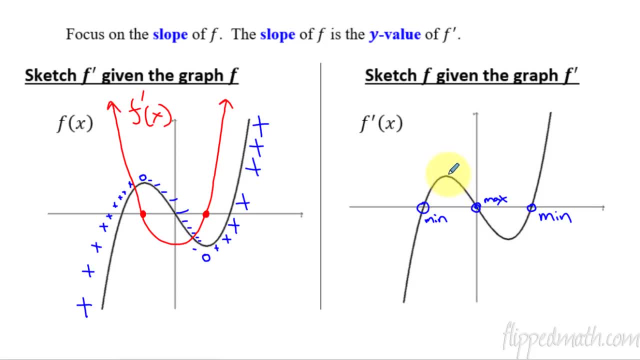 signs from zero. here it's zero, but it goes from positive to negative. so we know that this, right here, is a point of inflection. I'm just going to abbreviate here, because I'm going to end up drawing something, And we know this. 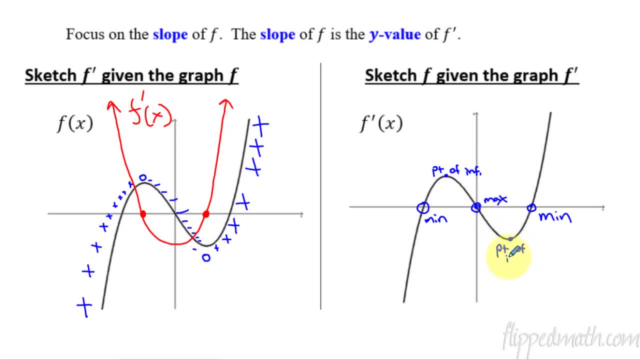 one is also a point of inflection. Oops, I know how to spell Okay, point of inflection. So now, what does the graph look like? Before I graph anything, I want to bring something to your attention and that is maybe on the side of your notes. 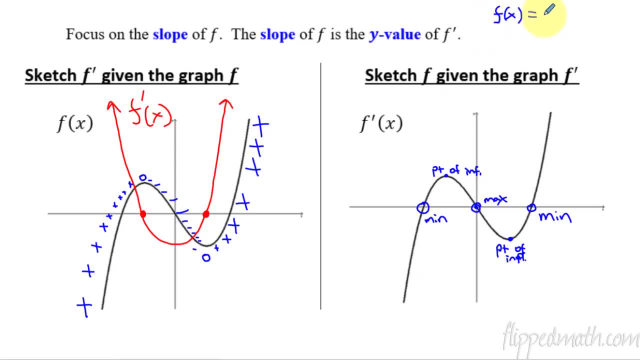 if you were to write, let's pretend like: f of x equals 3x squared minus 2.. The derivative of that is 6x, right, Okay, let's come up with another function: f of x equals 3x squared plus 1000.. The derivative of this one is 6x. 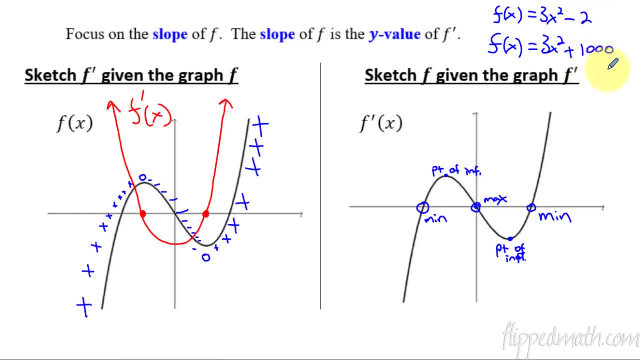 Both their derivatives are the same, but they are not the same graph. One of them is shifted 1002 units above this one. They're not the same thing. So what I want you to understand is that when we're going from f-prime back to f, there could be some constant at the end, Some plus a. 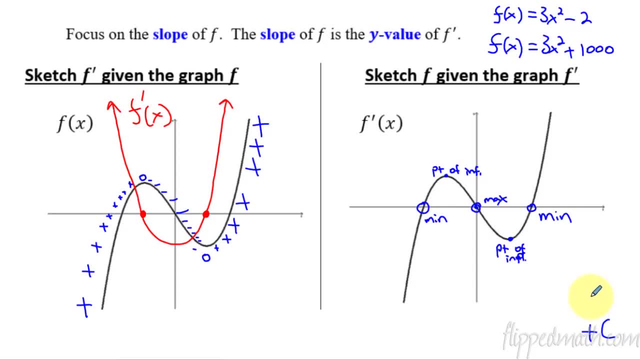 constant, I'll say a plus C, That we don't really know what. that is okay. So when you sketch f and all you have is f-prime, there could be an infinite number of answers if you just vertically shifted it up or down. So when you do the 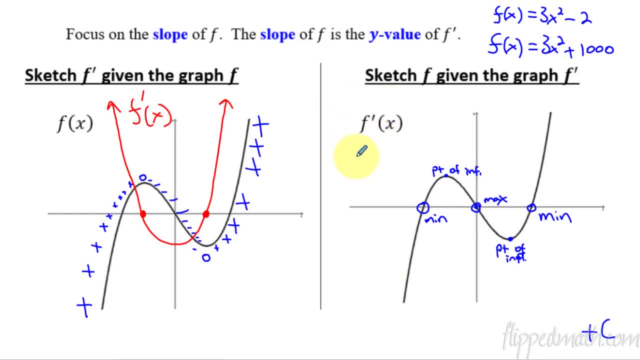 practice and you start with an f-prime and you're going back to f, recognize that it could be a vertical shift anywhere. It may not look exactly like mine, but the minimums, the maximums, the point of inflections, those are things that should stand out. They should be at the correct X value. 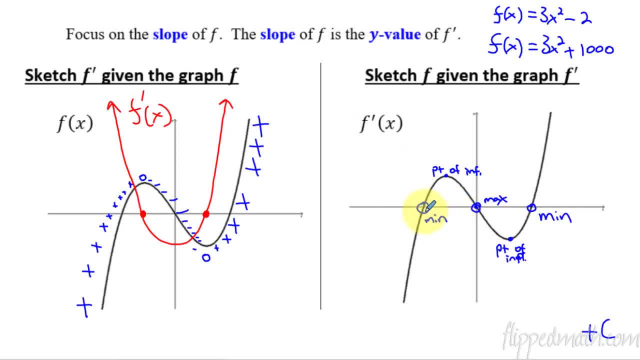 So let's try this. Let me switch my colors again. I know I have a minimum. Now where is the minimum? It could be anywhere, shifted up or down. I'm just going to put it right here. So I'm going to mark. 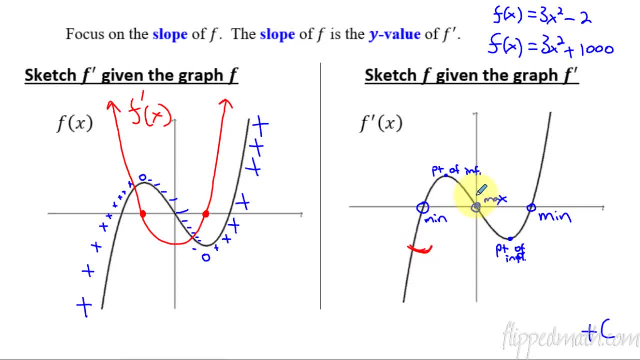 that I have a minimum here and just have it curve. here I have a maximum, so I'm just going to have it have a maximum up there where it curves. here I have another minimum, so let's have it curve down like this. And then what else do I know Points of inflection, So I'll put the point of inflection. 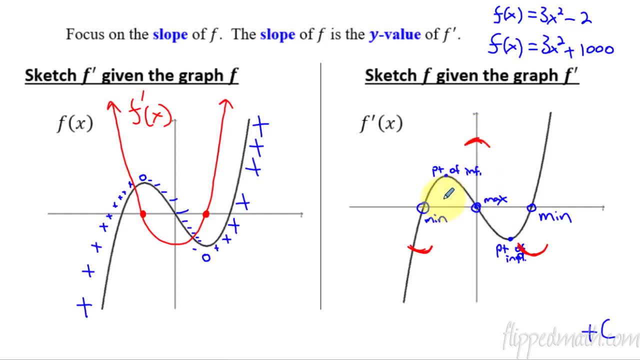 on this X value here, right in between the max and the min. So I'm just kind of eyeballing it here. I'm going to estimate about there And then my point of inflection on this X value: again, it's halfway from the top and the bottom of my graph, So I'm just guessing right about there. 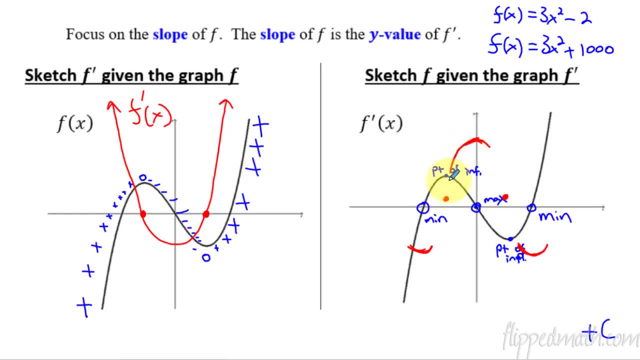 And now from here you can sketch the graph. So I have my maximum point, point of inflection. concavity changes. Now it's concave up, goes up forever and ever. And here I go down. Now the concavity changes. Let's go up to that point of inflection. 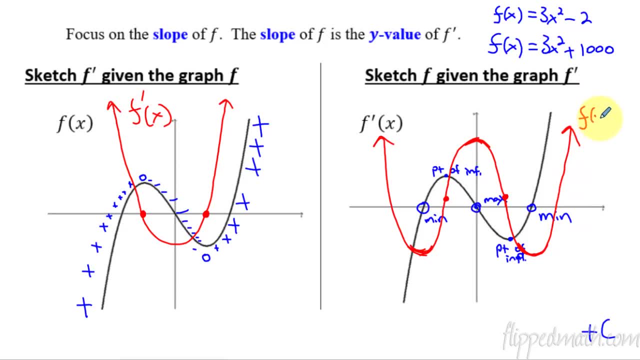 And then this one goes up forever and ever. So you have in red the F of X Again, this graph that's in red. it could be shifted all the way up, It could be shifted way down and it would still work. Obviously, you want to be able to graph it on the grid itself, But the important thing is that. 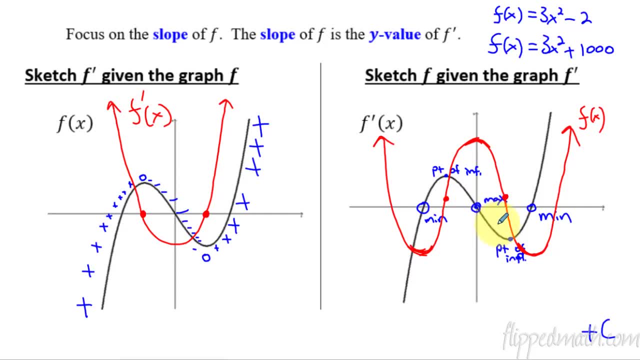 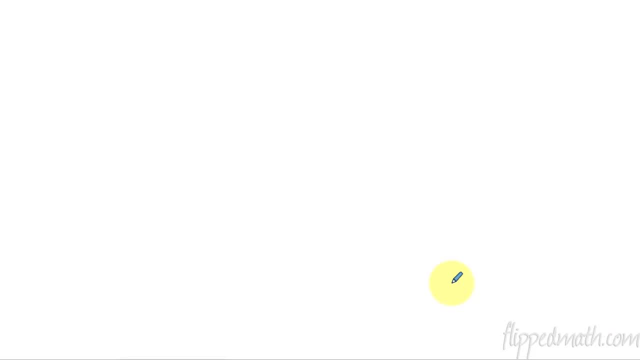 the X values of the min match up. the X value of the maximum matches up. the point of inflection should match up all of those types of things. Okay, before I close the video, let me just point out one more quick thing that can help you, And that is if you recognize certain patterns. 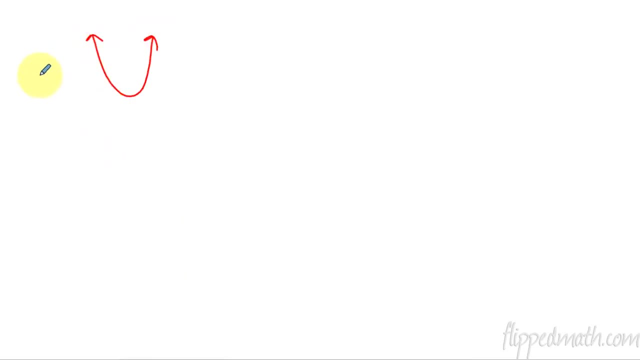 if I have a parabola- and you already know, a parabola is like X squared Well, the derivative of that is 2X. So the graph of 2X is just a flat line. So you could save yourself some time if you. 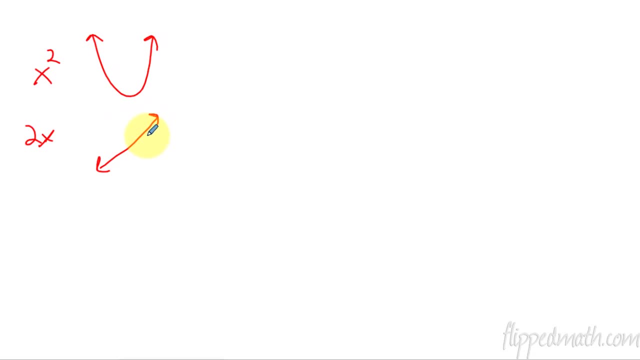 recognize a parabola's derivative graph would be linear. And then what would be the graph of that? A graph of a straight line would just be a constant. So that would be a constant at Y equals two. So there are little shortcuts that you can use, but you don't want to solely rely on that. 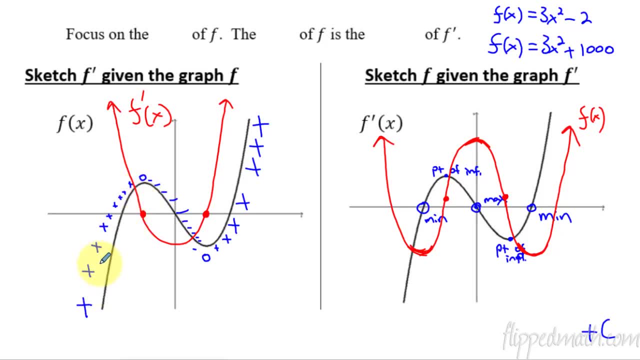 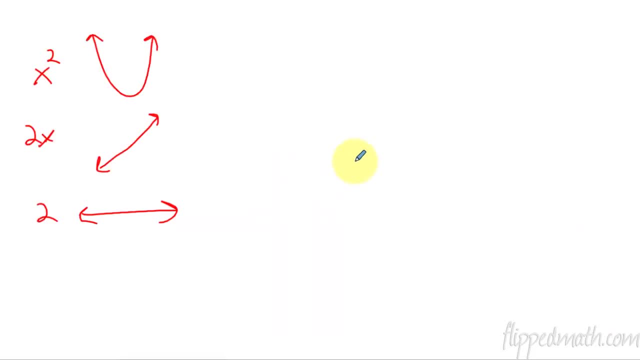 You need to be able to identify these little plus minus things when you're going from F to F- prime or the min and maxes- And the reason is because you will sometimes have a crazy problem. I'm just going to draw a quick grid. you might have a crazy problem that looks like this, And then we'll come. 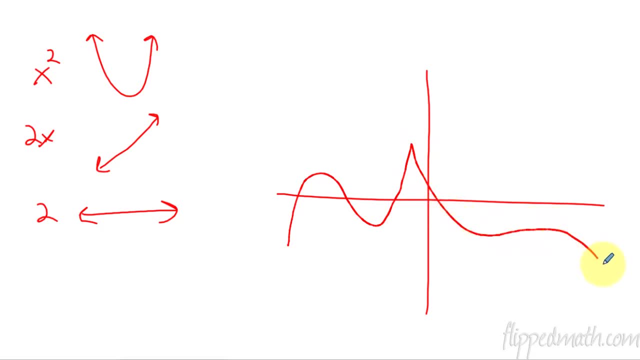 up, have that sharp corner, come down and then go down like that. Okay, now, if you had that, we don't have any rules that help us- just memorize that, like we had with X, squared and 2X. So you would need to identify again. this is I'm saying like that's F prime. you would need to identify. 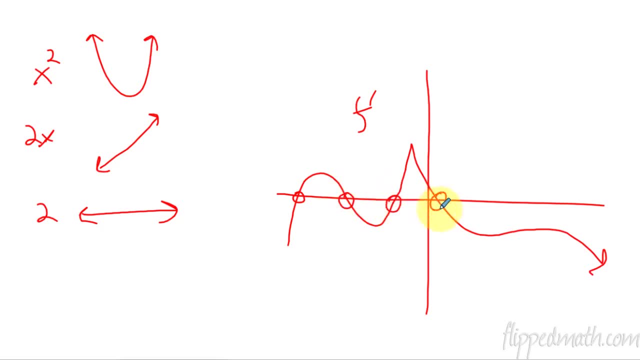 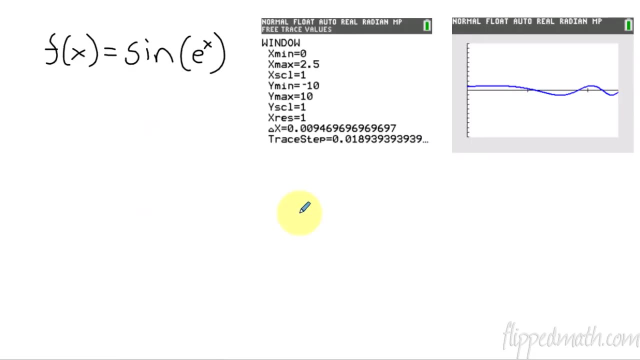 minimum maximum, minimum maximum- and then be able to try and very roughly sketch out what the graph of this would look like. Now I know I said I was almost done And I promise this time I'm really almost done. Okay, I do have another thing I got to talk to you about, But that's because 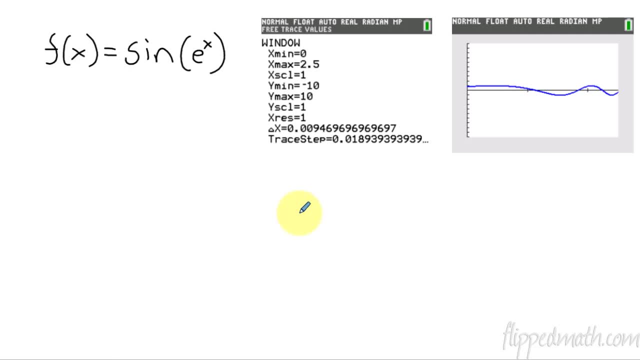 your calculator will actually draw the derivative for you And you don't even have to figure out what the derivative is. So I want to take this example we have. I have a function: F of x equals sine of e to the x. Now we could take the derivative, we could figure out what. 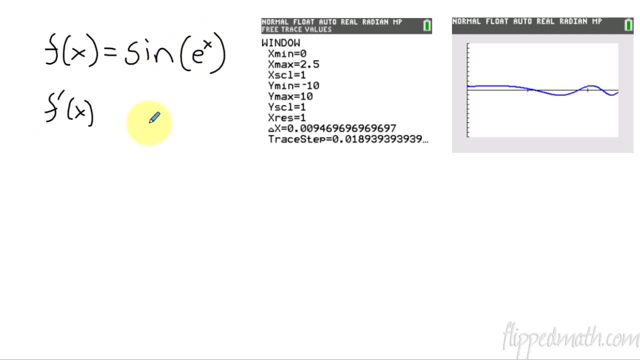 the derivative is by using the chain rule. cosine and use the chain rule stuff. It's that this is not too hard, difficult of a problem, But I want to show you that the calculator can do it for us and just graph the derivative. So here I've set up my window And if you want to grab your own, 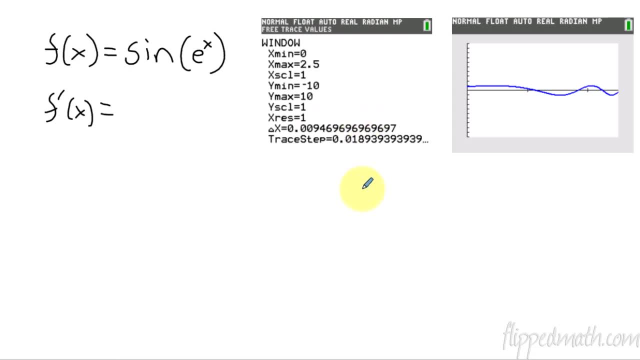 calculator, just to practice. this might be a good idea, just to make sure you can do this. Again, if you don't have a TI 84, you'll have to look up how to graph the derivative. some instructions on how to do that. So I've got my zero to 2.5.. I've got my min and max scale, all this stuff. So this: 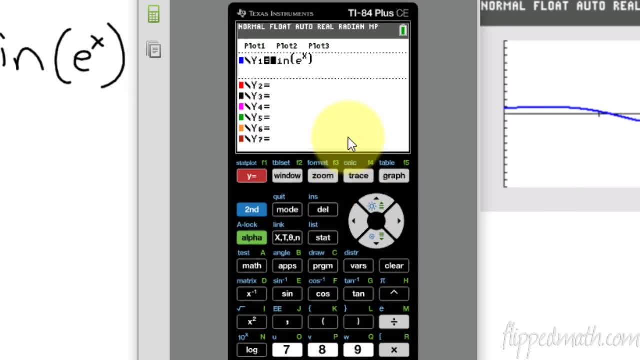 is what the graph looks like. Now here is what I would do for graphing the derivative. I'm going to take my calculator and I already have my y equals, blah, blah stuff in here: sine of e to the x. And now, on the second line, I would like to graph the derivative by: for a TI 84.. It's the math button. 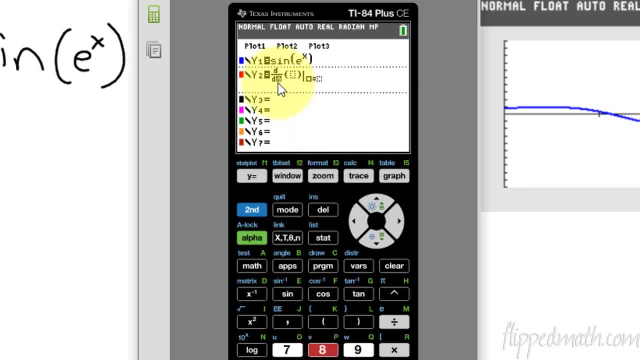 and then option number eight. option number eight is the derivative, So math eight. And now I have set up, I'm going to take the derivative with respect to x, I'm going to type in sine of e to the x, just retype it. Or I could say: I want the variables. 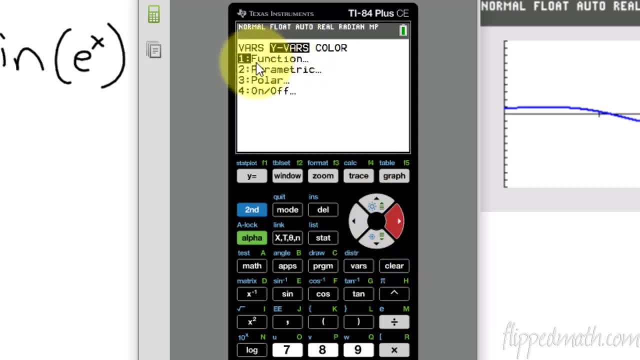 button, the y variables go over. I'm doing function number one and I want to type in whatever I have in y1. So now what that does is that gives me the derivative of the function that I typed out into y1, the line y1. And now, at x equals. and what we've done before is we've said: 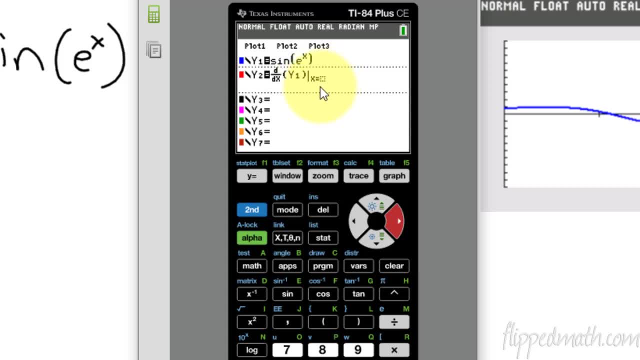 the derivative at a specific point. So we'd say like x equals two, and we'd spit out a number. But now in this case, what I'm going to say is: I want the derivative at x equals x. What that means is I'm going to take the derivative at every single possible value of x and then I hit graph. 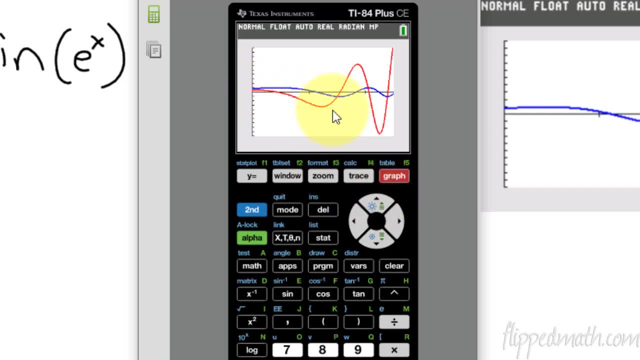 Now watch what happens. Sometimes it goes really slow as it has to calculate what the derivative is, But in this case you now can see this red line that is the derivative of the original function. Let me copy this over to my page, So now you can see here the original function in blue.